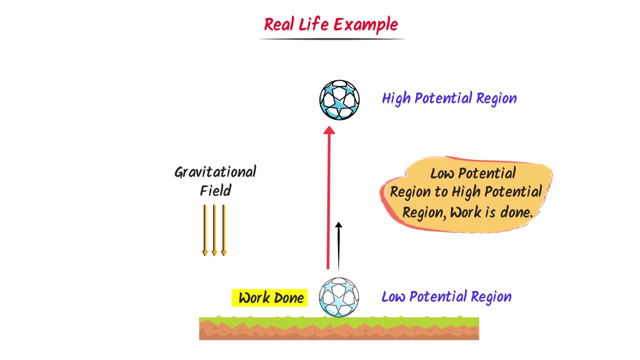 potential region and gravitational field, we need to do some sort of work on the object. Let me repeat it: If we want to move an object from low potential region to high potential region and gravitational field, we need to do some sort of work on the object. Secondly, when we do some sort of work, 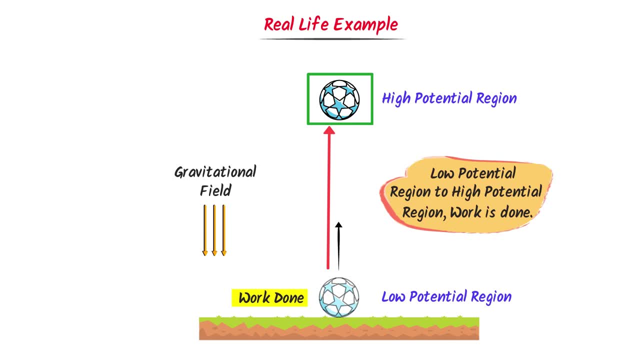 on the ball against gravitational field. as a result of this, this work done is stored as potential energy. So the second fact is, when we change the position of an object in gravitational field an opposite direction, then the ball moves down As a result of this. 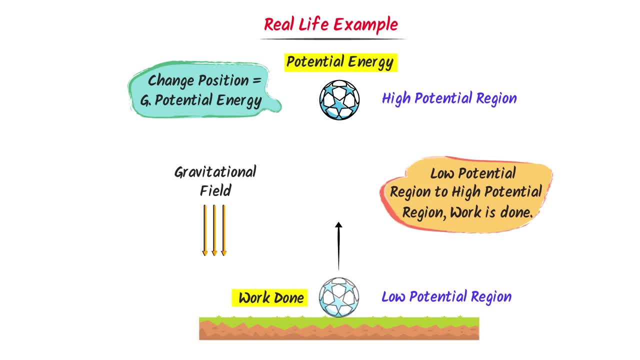 we get the result. Now let us see how can we change this one. Well, in this study we have direction. gravitational potential energy is stored in the object. Let me repeat it: When we change the position of an object in gravitational field in opposite direction. 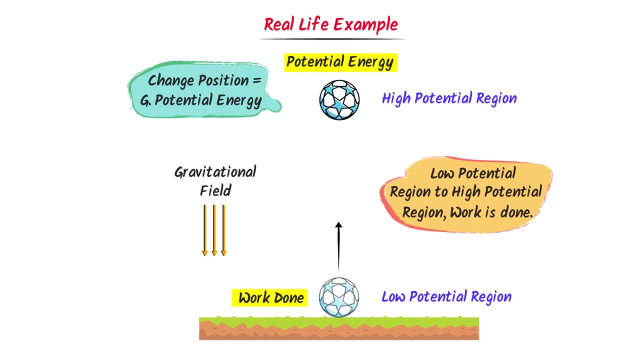 gravitational potential energy is stored in the object. Finally, if I release this ball from high potential region, it will accelerate towards the ground. Here is one very, very important point: When this ball falls from high potential region towards low potential region, it possesses kinetic energy due to its motion and we can utilize its kinetic energy. 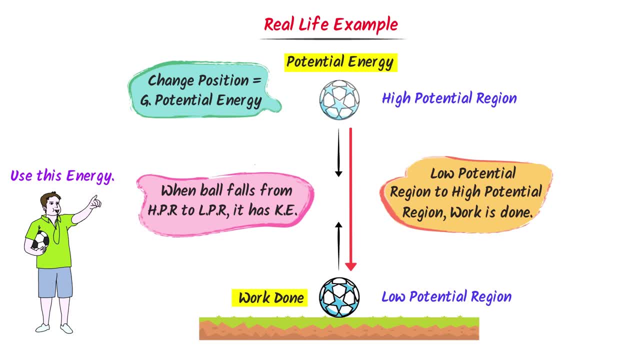 Let me repeat it: When this ball falls from high potential region towards low potential region, it possesses kinetic energy due to its motion and we can utilize its kinetic energy. So the third fact is Objects fall from high potential region to low potential region due to potential energy. 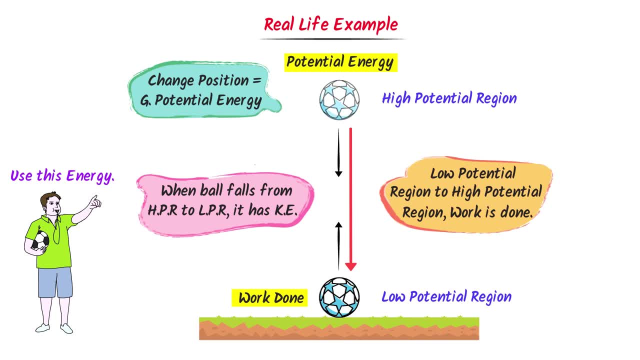 and we can utilize their energy. To conclude this slide, we learn three important facts. Firstly, we need to do some sort of work in order to move an object from low potential region to high potential region. Secondly, when we change position of an object in gravitational field, gravitational potential- 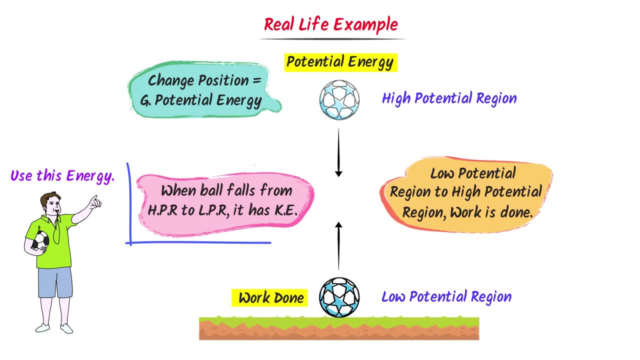 energy is stored in the object. Thirdly, when object falls from high potential region to low potential region due to gravitational potential energy, we can utilize its energy. Thus, using these three facts, we can easily learn the concept of electric potential. Now, what is electric potential? 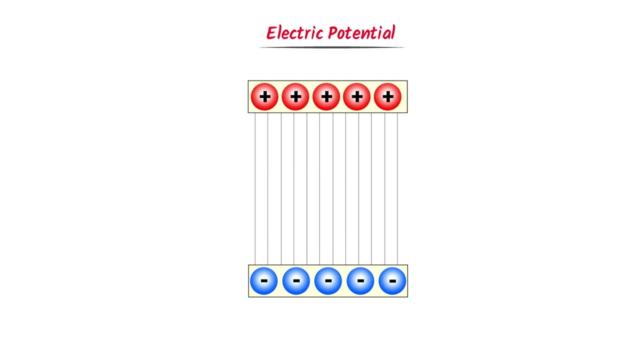 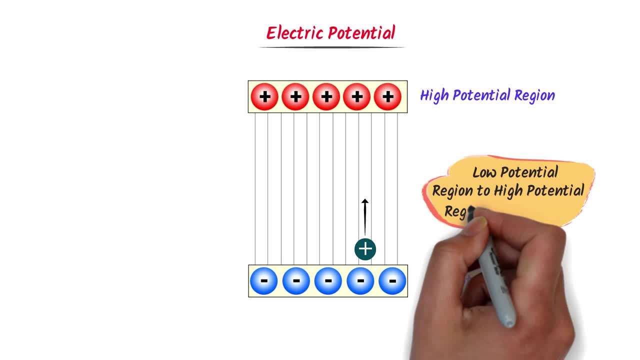 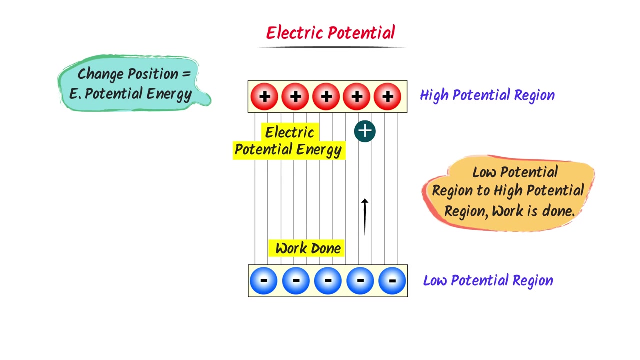 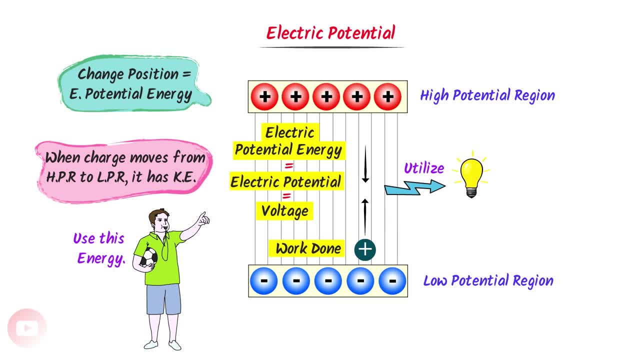 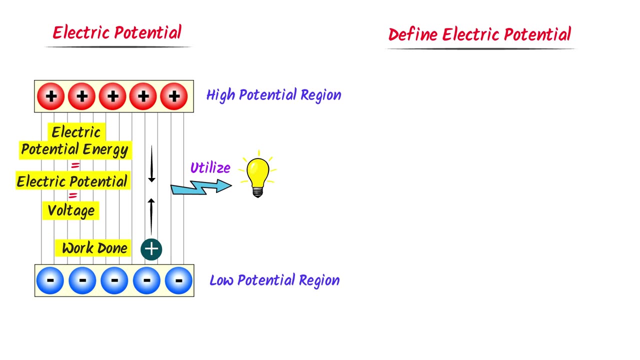 to low potential region. we utilize its kinetic energy to light a bulb, So remember that we can utilize the electric potential energy of this test charge. Now, how can we define electric potential? Well, let me explain it in a very simple way. Firstly, we do some sort of work on the test charge against. 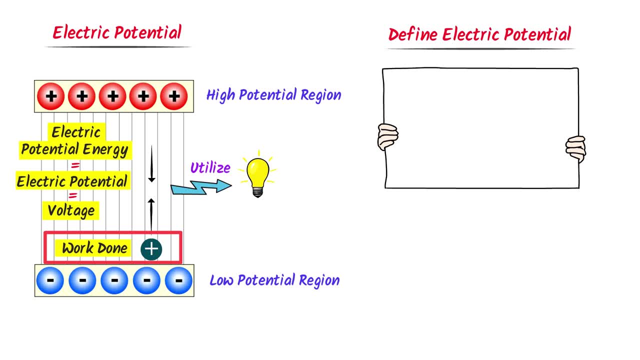 electric field. Secondly, as a result of this work done, the position of test charge is changed and electric potential, energy or electric potential is produced in the test charge. So it is the work done on test charge that is generating electric potential. Let me repeat it: It is the work done on test charge that is. 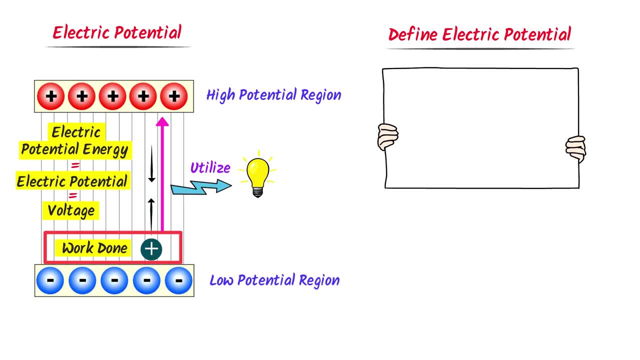 generating electric potential. Now, if I do not do some work on this test charge against electric field, then how can we define electric potential In the test charge? its position in the electric field will not change and no electric potential is generated. Therefore we define electric potential. 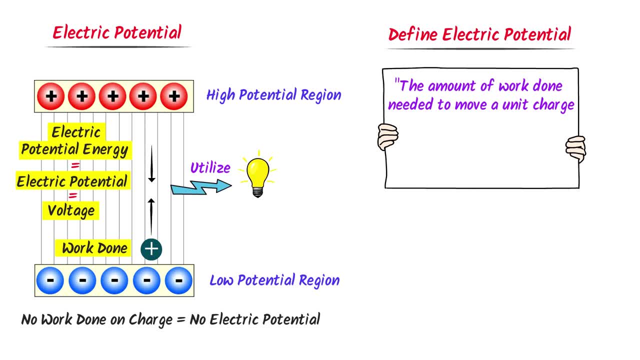 as the amount of work done needed to move a test charge from a low potential region to a high potential region against an electric field is called electric potential or voltage. Or simply remember that electric potential or voltage is equal to electric potential or voltage. So electric potential or voltage is equal to work done per unit charge or v is equal. 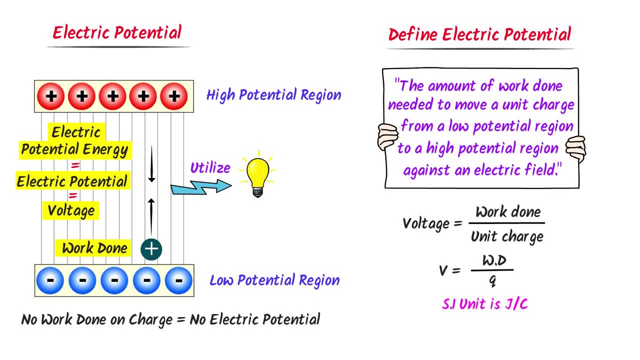 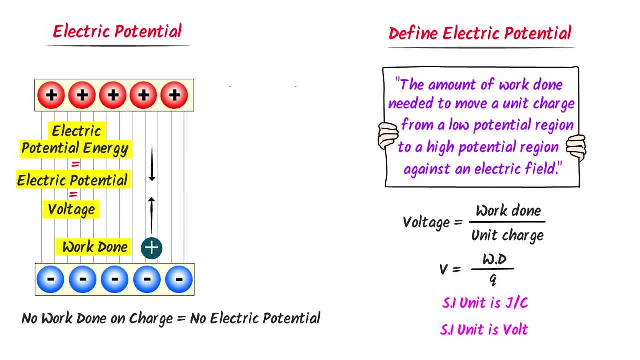 to work done on q. The s unit of electric potential or voltage is joule per coulomb or simply volt. Here let me teach you one of my favorite questions. We know that electron is extremely small, which we cannot touch or see. So how can we do? 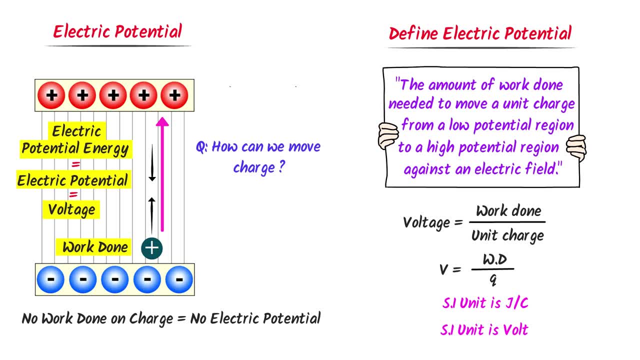 some sort of work or move this electron and electric field. Well, we use emf or chemical battery to derive this electron from low potential region to high potential region. So emf or electromotive force is nothing, but it derives electrons from low potential region to high potential region, Or we can say that it keeps the constant.